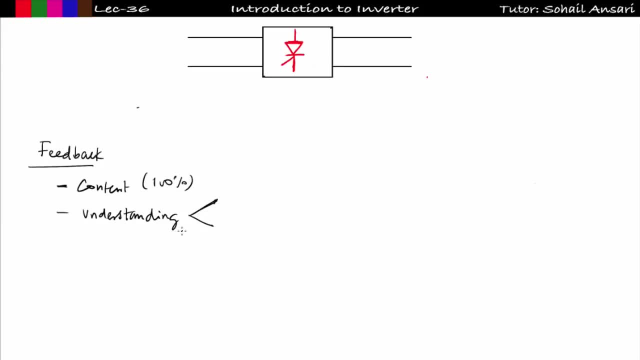 the concept or not. I need the feedback of this. If you are not understanding, tell me in the comment that you are not understanding. So how will you give feedback in terms of like, in terms of dislike and in terms of comment? If you are not understanding the content given by me, then please hit dislike. so 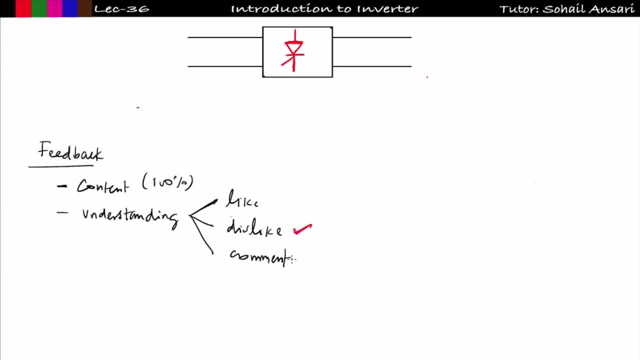 that I would be able to understand that whatever I am providing you- that is trend- are not understanding. Okay, so I will make. I will try to make a next video in another way. Okay, so hit dislike there is a video, then I will stop making the video. that is not like that, because everybody is having their. 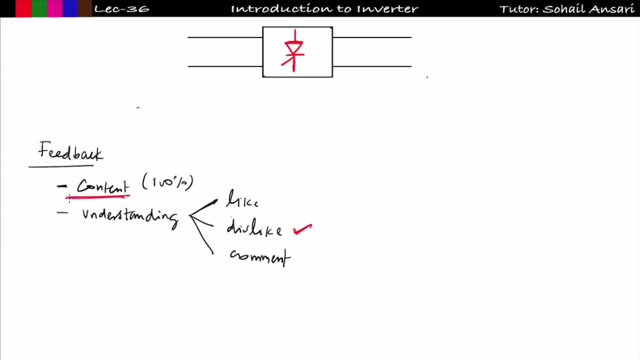 own opinion. so I am not fear of getting this like because I know, whatever the content I am providing you, that is 100% strictly related to get. Okay now, if you understand the concept, then hit like and also comment below why I am telling you to comment. you should comment that, sir, I understood. 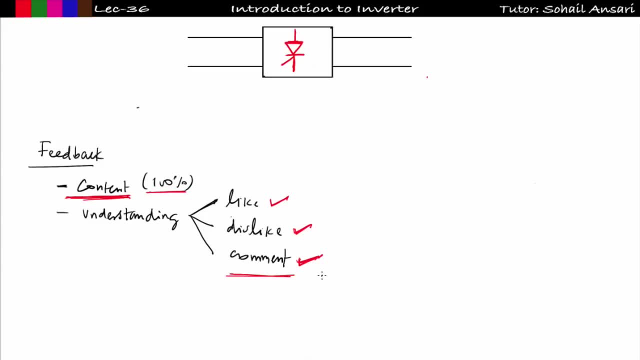 each and every concept. Okay, if you will not do this, then how will I able to know that, whatever the content I am going to give, to give you that students are watching? so if you will not watch the video, if you will not give me the feedback, then how will i make the next video? this is not like one-to-one conversation that i 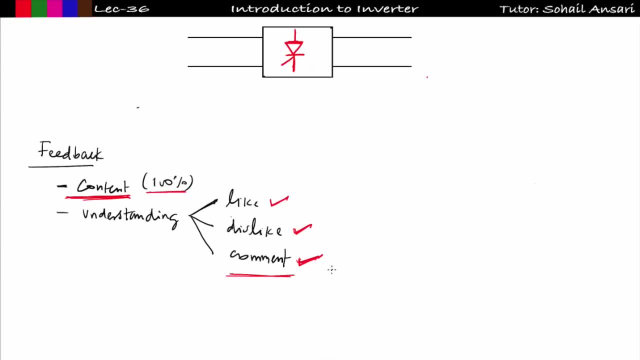 am delivering the video you are storing in your folder and you are not watching. so what is the benefit of that if i am putting this much of effort and if i am giving you the free content by putting this much of effort? you should like or dislike or comment. i just want the feedback from. 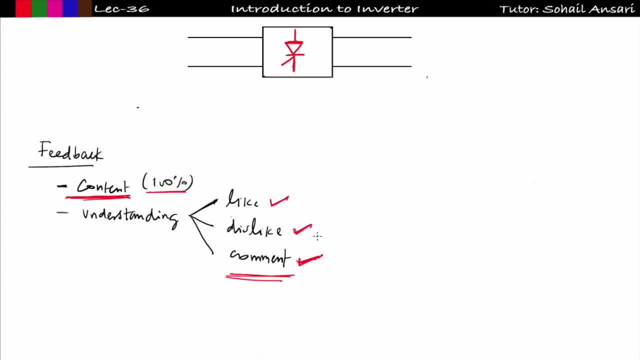 your site. if you are watching this, then hit like or dislike or comment. if you are not understanding, tell me in the comment. i am not understanding. that's why i am disliking your video. okay, so after this lecture, i just want to say that please give me the feedback whether you are capable of. 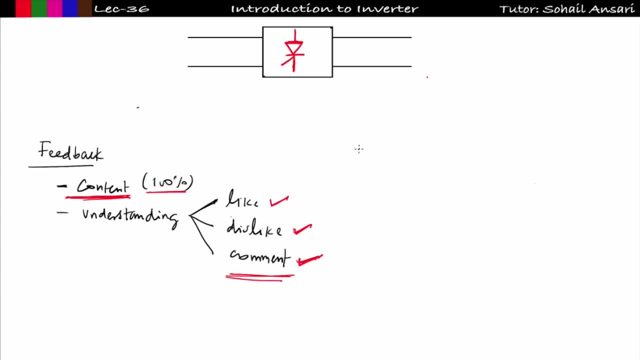 understanding my concept or not, got it. now, from this lecture onward, i will include one more features in video. that is homework. some of the students told me that you should provide. you should give one questions related to your content. so i will include one more feature in video that is homework. some of the student told me that you should provide. you should give one questions related to. 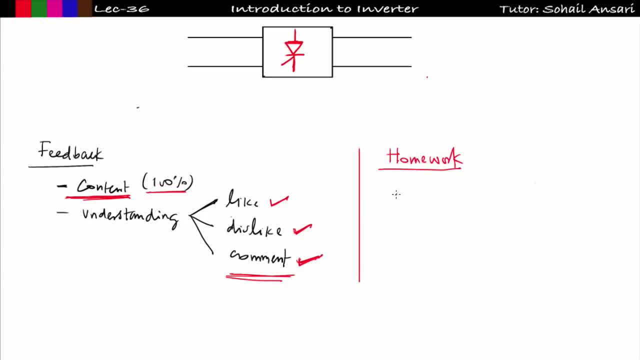 that lecture so that it clears the concept in detail. so after completing each video, i will give you one homework and you have to solve that questions and you have to comment the answer of that question in youtube comment. okay, even if you are downloading the video, then watch the video. 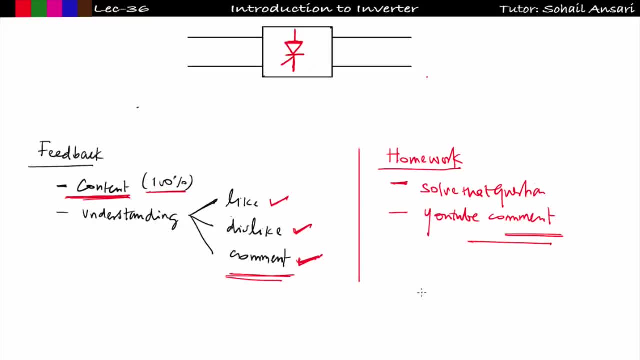 no problem. share the downloaded video with your friends, but try to read those concept and try to solve this homework, and please give me the answer of that in youtube comment. this is really important for me. it will motivate me to make the next lecture. got it? so please take this seriously. 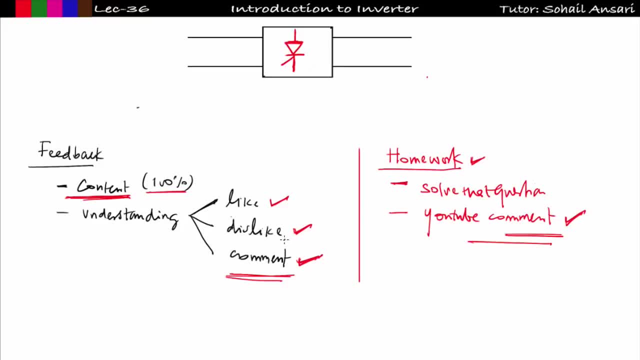 because i want a feedback from your side. if you are watching the video, if you are understanding the concept, then please hit like and also comment below that, sir, i understood the concept. if you have not understood the concept or you are thinking that you are not getting what i am telling you, 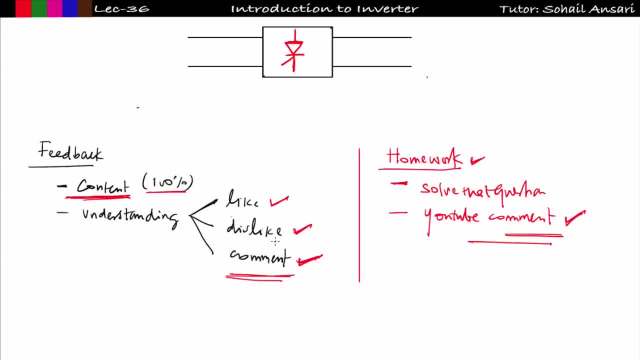 then write that problem in the comment below and you can hit dislike also. there is nothing to worry about. youtube has given you the like and dislike as well, so no need to worry about got it now. let's now start this lecture. that is the introduction to inverter. 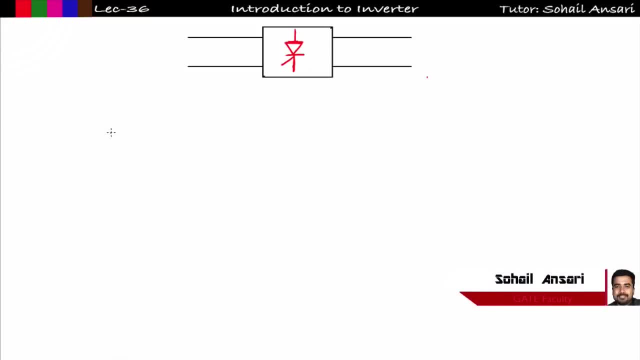 till now we have completed the rectifier which converts ac to dc, chopper which converts dc, fixed dc- to variable dc. now we are going to see the inverter. what is inverter? so inverter is another kind of power electronic circuit which converts fixed dc to variable ac. voltage means it is a dc to ac converter. now, if i will talk about the fixed, 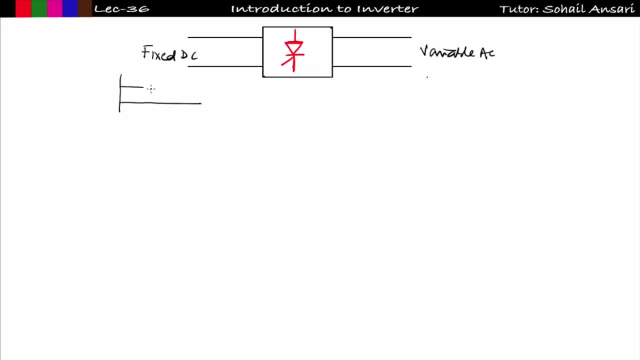 dc, then the fixed dc will look like this: this is my fixed dc having some peak value. let us say this is vdc now at the output of the inverter, which type of waveform i am getting? i am getting like ac waveform, like a square wave having time period t, and it has some peak magnitude. that is vdc now. i. 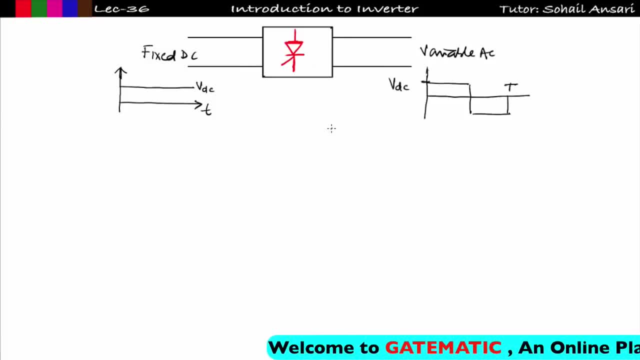 told you that inverter is another kind of power electronic converter which converts fixed dc to variable ac. so what do you mean by this variable? variable means we can vary the magnitude as well as we can vary the frequency. so first talk about how we can vary the frequency, like i want at the 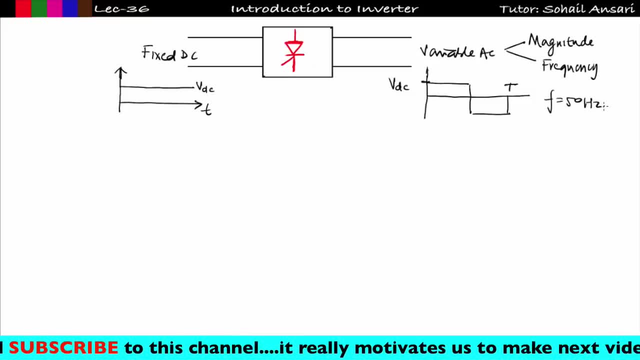 output side the frequency must be 50 hertz. we know in india the frequency is 50 hertz means the time period will be equal to 1 by f, that is equal to 20 millisecond. so by varying the switching of this power electronic devices we can vary the time period. but how will i vary the magnitude? 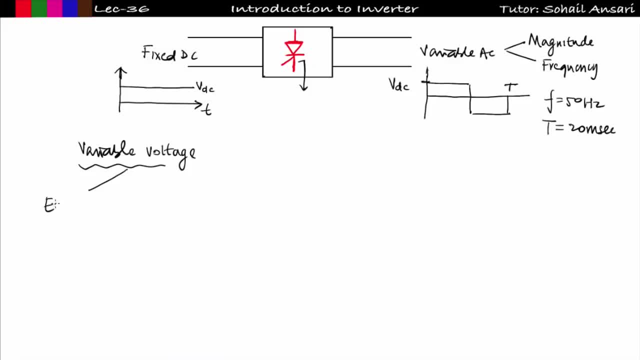 in order to get the variable voltage, two process is done. first one is the external control and second one is the internal control. internal control means we can control the rms value of voltage by pwm technique. these all things we will see. an external control means we will insert. 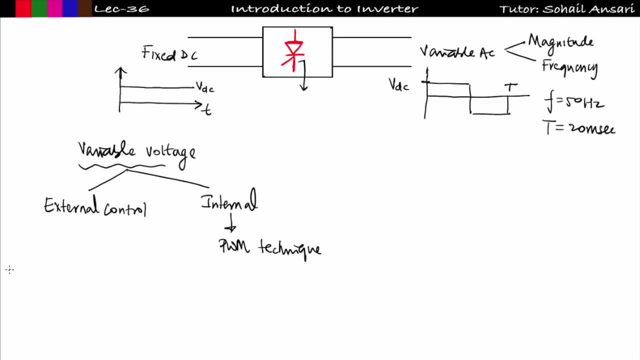 another kind of converter which will produce a variable dc and then we will control the. and by producing variable dc we can make the variable ac like. i will take ac input and i will pass this ac input to control rectifier. so if i'll pass this ac input to control rectifier, then i will 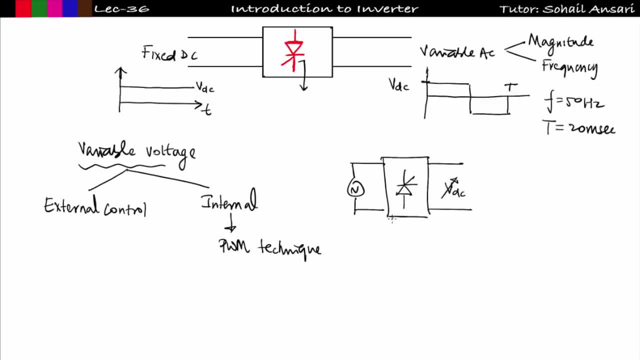 get here variable dc, okay, which may vary, and the value of vdc we can control by varying alpha of this rectifier. now, this variable dc i can give to inverter, okay, second way to control the dc voltage, that is, i will include dc to dc converter, whether it is buck converter boost. 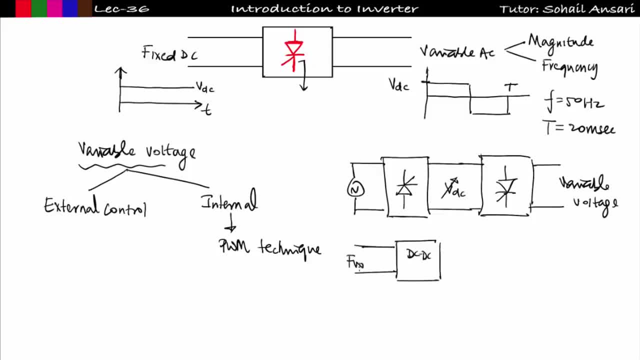 converter or dc buck boost converter. i will take this fixed voltage here. this converter will give me the variable voltage and that will be dc. okay, and now this variable dc voltage is given to the input side of inverter to get the variable ac output voltage got it. these are some a process. 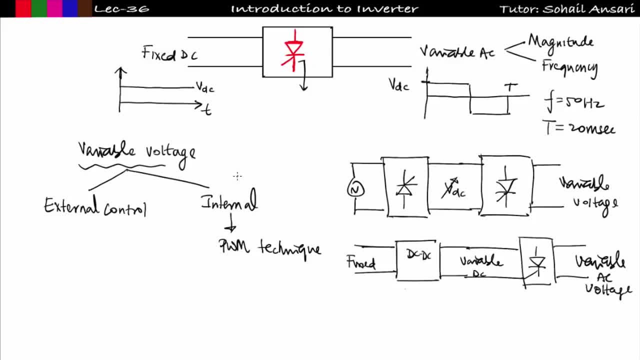 of controlling internally as well as externally. internal control we will see later on. that is the pwm technique. now the problem is if i will give the fixed dc to the inverter circuit, then at the output we are getting the square wave. but what i want? i want that. 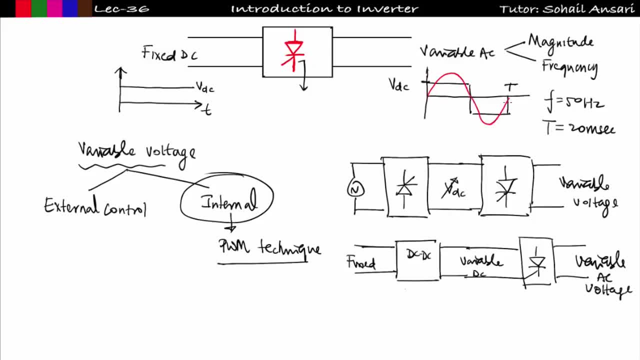 the inverter must produce the sinusoidal wave like this. so can i use this circuit for real time application? no, we cannot connect this circuit for real time application because at the output of the ac side we are getting a square voltage, not the sinusoidal voltage. so this is the problematic situation for any power electronics design engineer. 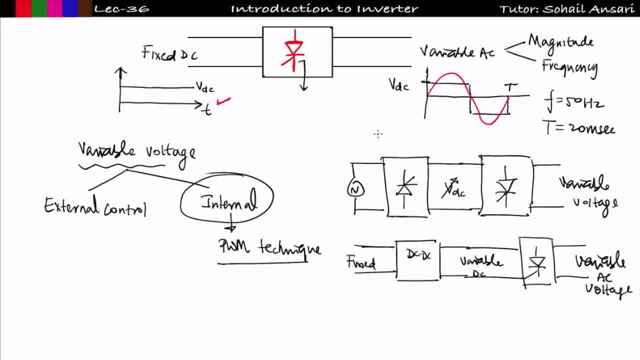 okay, we cannot connect this circuit or this inverter to real time application, then what is the purpose of making the inverter? we need, at the output side, pure sine wave, but at the output side we are getting a square wave. therefore, it is very much necessary to analyze the fourier series. 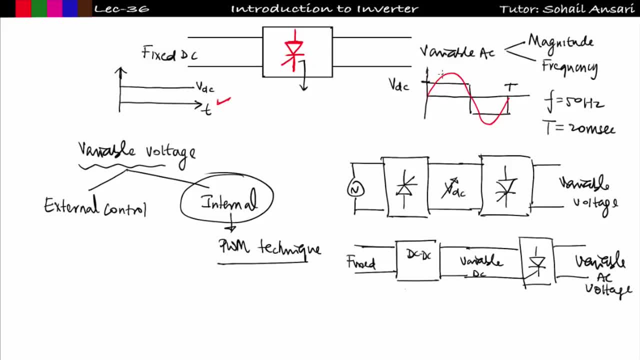 of this square wave because at the output side we need only fundamental frequency, that is, the sinusoidal wave. so in order to get the sinusoidal wave, we need only fundamental frequency, that is, the sinusoidal wave. so in order to get the sine wave, what we do, we will do the fourier analysis of this square wave. this is: 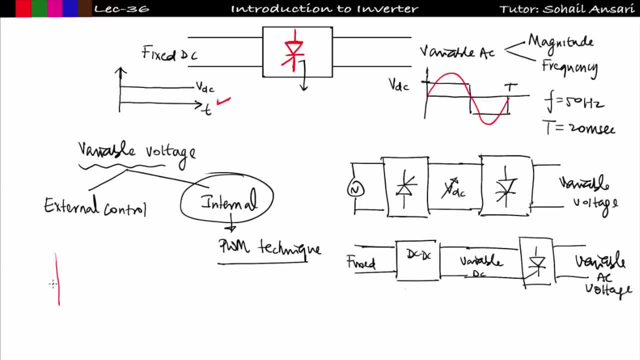 very important for design engineer. so what i will do as a design engineer, i should analyze this square wave in terms of sinusoidal wave. this is my desired wave and this waveform i am getting at the output of inverter terminal. so let us analyze the fourier series expression of this square wave. 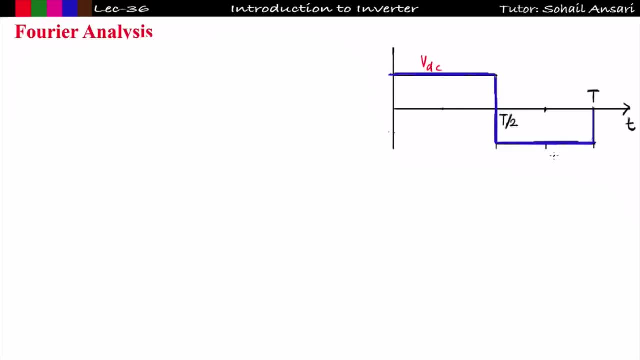 let us take the output voltage. so let us take the output voltage having peak magnitude, vdc, and here it is having minus vdc. then if you will do the fourier series analysis of this v, not of t, let us say this is the output waveform, then it contains the odd harmonics. n is equal to. 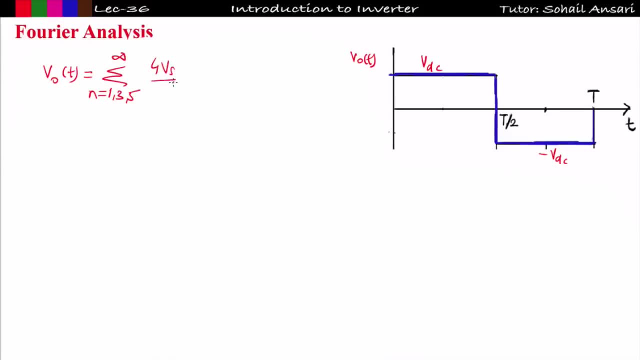 1, 3, 5 to infinite 4, vs upon n, pi sine n, omega naught t, where omega naught is the fundamental frequency. now most of the students are having a fear of four-year series, so it's very powerful. so in order to solve the problem, dots the fourier series, we need to 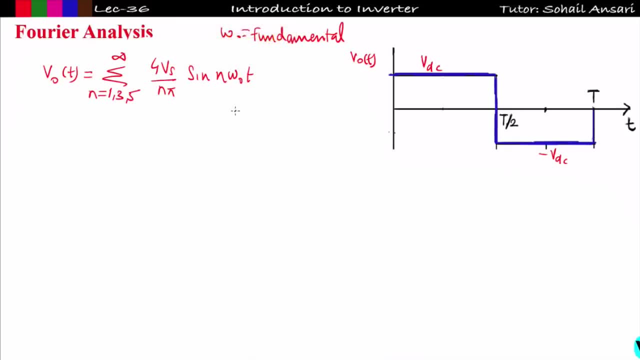 find the number qualification of the signal wave. also, what you can do is calculate in the plus 4 vs upon 2 pi. this will be not 2, this will be 3 sine 3 omega naught t plus 4 vs upon 5 pi. 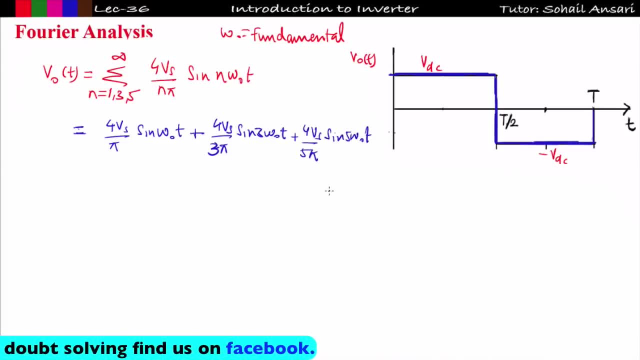 sine 5, omega naught, t, where omega naught is the fundamental frequency, and so on, and this is my v? naught of t, which we are getting at the output of the inverter terminal. now let us analyze this by waveform. i can say this is something like this: this is my square wave, and this square wave is: 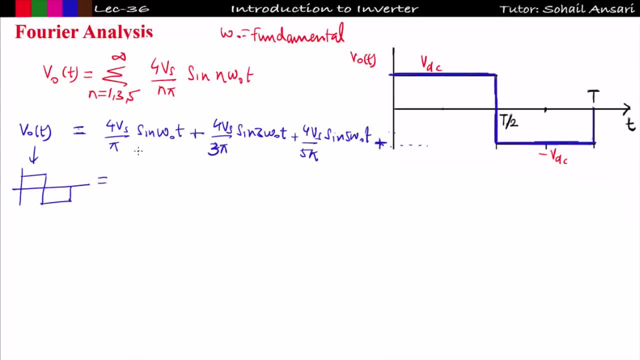 converted into series of sine wave having different frequency. so this is my fundamental frequency. so it will look like this: having time period t: this is also having time period t. now draw the third harmonic component. third harmonic component will look like this: this is my time period. now draw the fifth harmonic component. fifth harmonic component will look like this: 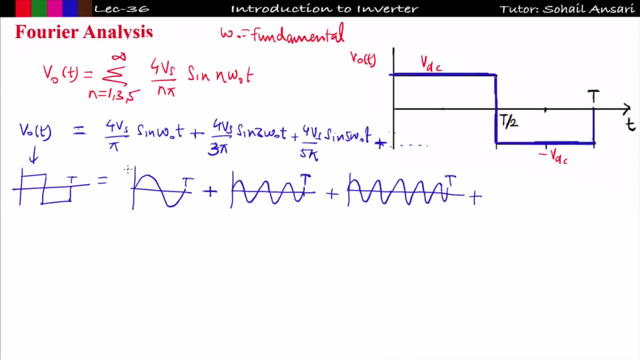 is it fine? so a series of third harmonic, fifth harmonic, then seventh, then ninth, up to infinite. is it fine? so a series of third harmonic, fifth harmonic, then seventh, then ninth, up to infinite will give me this square wave. what do you mean by this? this means, if i will add the fundamental, 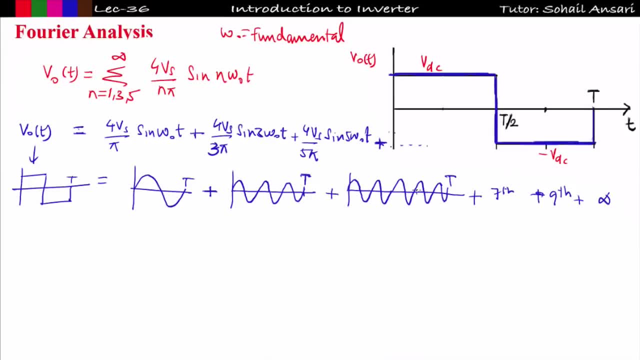 sine wave, with third harmonic sine wave, with fifth harmonic sine wave and so on. then the output waveform i will get, that is the square wave. are you getting this? so here comes the analysis of fourier series. why we are doing the fourier series analysis in inverter as a design engineer, what we 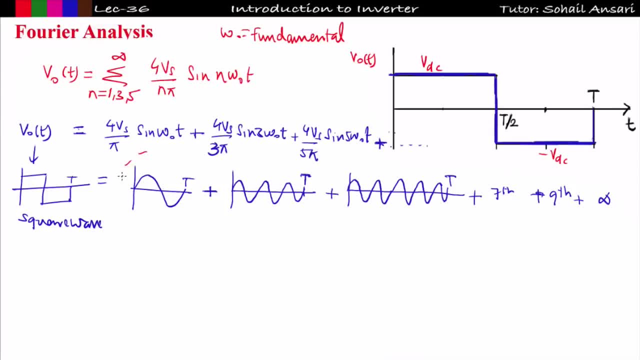 want at the output terminal. we want at the output terminal this one. this is my desired waveform, but because of a square waveform we are getting the harmonic component, that is, a third harmonic, fifth harmonic, seventh harmonic, ninth, harmon up to infinite. because of that, we are getting the square waveform, so any square periodic waveform can be. 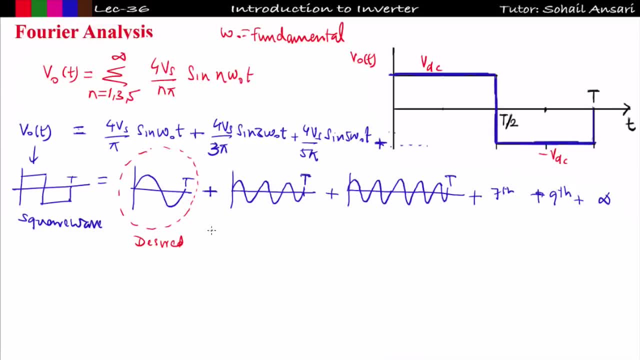 resolved into a sine waveform having different frequency. so, as a design engineer, what i will do? i will keep this waveform and i will remove the other waveform. if i will remove this all, then at the output of the inverter i will get only fundamental sine wave, and this is my desired. 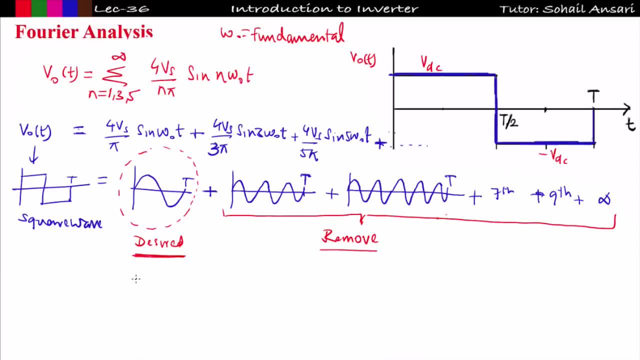 waveform. so that is why a power electronic engineer analyze the fourier series operation, so that they can separate the fundamental sine wave from other way. so these all wave are known as harmonic component and as a power electronic engineer we should not have a fear of harmonic. what is harmonic? harmonic means non-fundamental component of current or voltage. so he 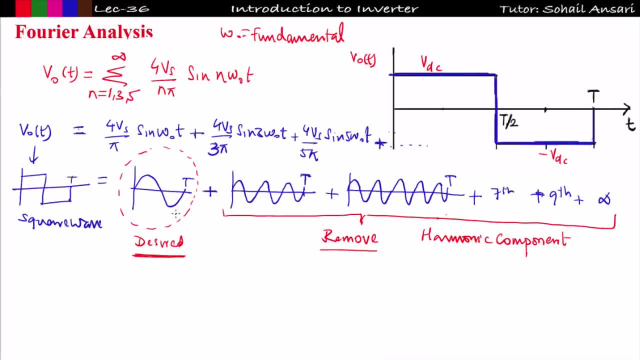 so here the fundamental component of current or voltage. I am getting at a starting. so whatever the waveform left, that will be the harmonic component. this all concept I have given you in lecture number one of power electronics, how this 4 Vs upon n pi are coming, that is, 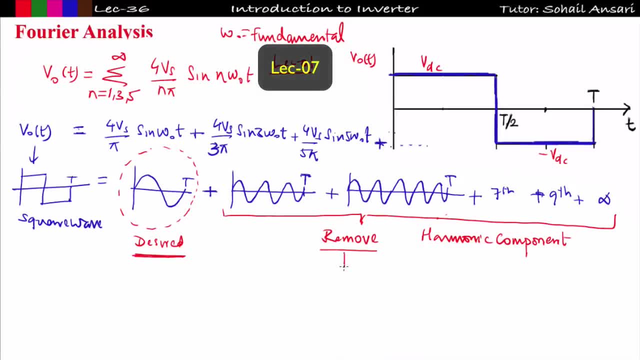 given in lecture number one. go through that. so to remove these all harmonic component, what we will do? we will attach filter circuit in inverter or we can make PWM inverter. okay, so by PWM technique also we can remove these all harmonic component. why this is necessary? 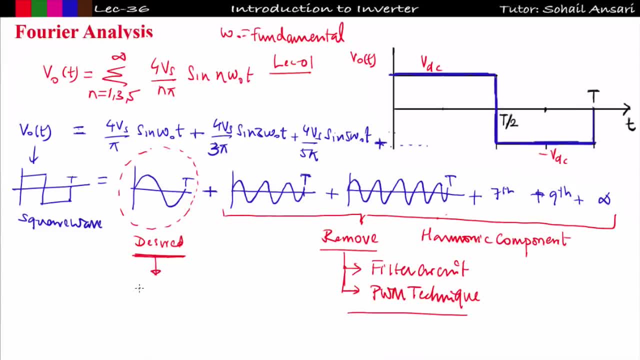 to get the desired output voltage, that is, the sinusoidal voltage. our aim is to get the sinusoidal voltage. so, while making the inverter output voltage waveform or output current waveform, what I will do, I will make this fundamental waveform also so that you should understand how much deviation is there. okay, so I will make this fundamental waveform also whose? 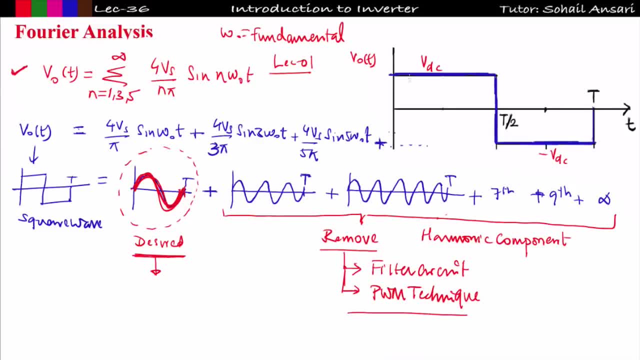 time period is a few seconds will be same as the square wave time period. so here a square wave is something like this. so fundamental waveform of this will look like sine wave and it will be something like this: in each of the inverter lecture i will make the fundamental. this is my fundamental waveform: v01t. 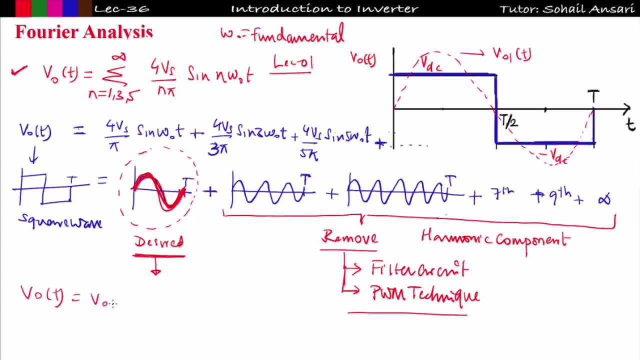 i can write: v naught of t is equal to v01t plus v02t. no, this will not be 2 because it contains only odd harmonics plus v05t and so on. i don't want to draw the waveform of these all things. 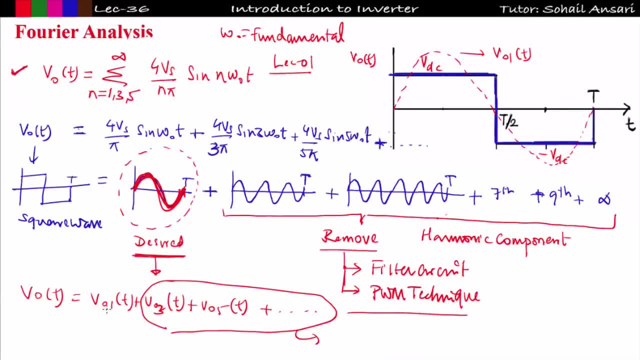 because these are the harmonic component which i need to remove. but i am interested in this waveform that is the fundamental waveform. so in each of the inverter waveform i will draw the fundamental waveform so that you should understand how much output voltage and output current are deviating from its fundamental. you should know this. now. there are some parameters. 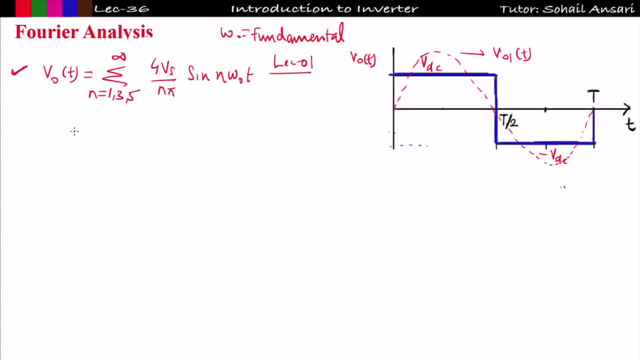 which in which we need to define, if i will talk about the fundamental waveforms, and this will be the fundamental waveform. so in each of these two cases, we need to define these 3 harmonics. that is, let us consider this v? naught of t, which is a combination of v01 of t plus v03 of t. it contains third harmonic plus v05 of t, and so on. 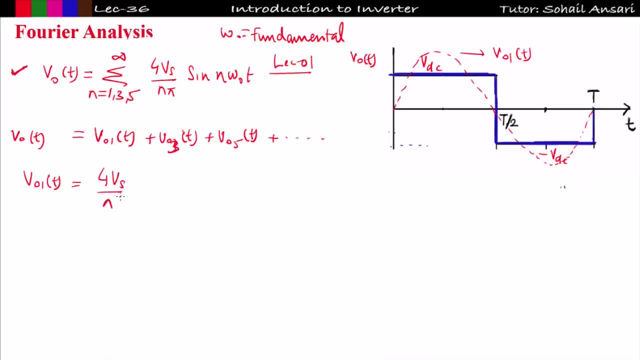 now, if i need to find the v01 of t, what i will do, i will put n is equal to 1. i will get the v01 of t, that is 4 bs upon pi sine omega naught. t where omega naught is the fundamental frequency. 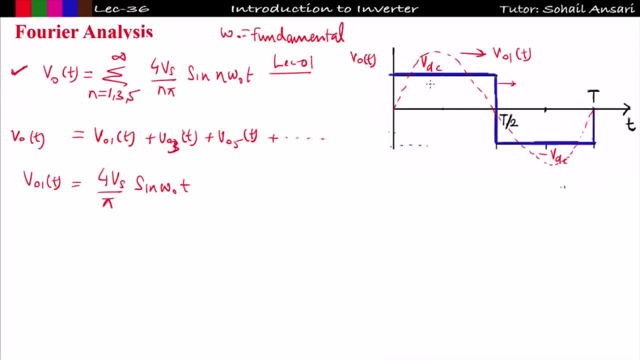 drawn here. this is the v01 of t. this is the total voltage waveform and this is the fundamental voltage waveform. are you getting this now? if i will talk about the v01 rms, then it will be. we know rms value of sine wave is equal to maximum value upon root 2, so it will be equal to 4 vs. 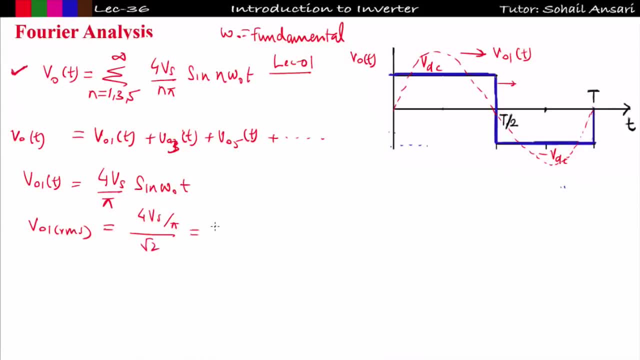 upon pi divided by root 2, i will get 2 root 2 vs upon pi. now what will be the total rms output voltage? see, this is the square voltage and i need to find the total rms voltage of this output voltage, which is square, wave. i already explained you how to find the rms value: square, the waveform. 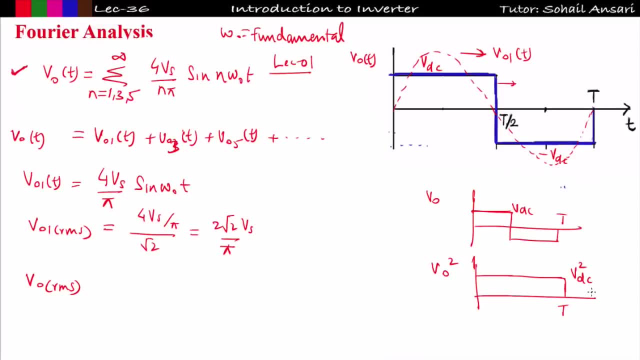 now find the average average you will get. that is vdc square only, vdc square into t upon t. that will give you the average. then take under root of this waveform so it will be equal to v0. rms is equal to under root of vdc square. that is equal to vdc only. so rms value i will get. that is equal. 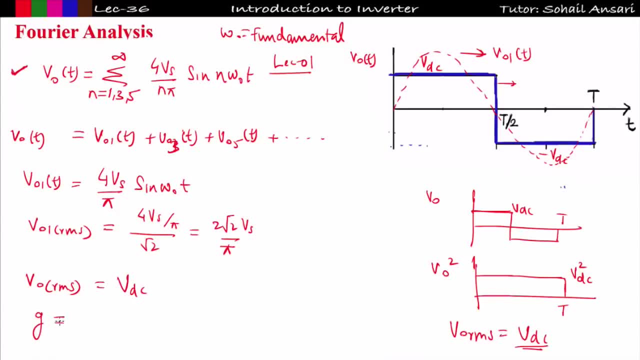 to vdc. so is one parameter defined in ac, that is the distortion factor. that that i have already explained you in the first lecture: v01 rms upon v0 rms, that you will get 2 root 2 upon pi. divide this equation and this equation, you will get this okay. so distortion factor is independent. 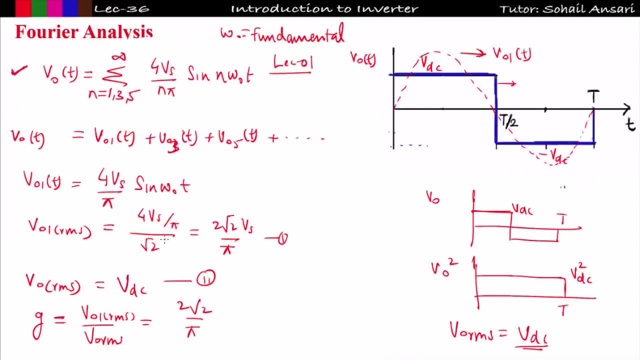 of the peak value of output voltage, see vdc. and vdc is getting cancelled out. let us consider that the vs and vdc are equal. that is the peak value of voltage. so after finding the distortion factor, i can say that distortion factor is independent of the peak value of output voltage. okay, and if? 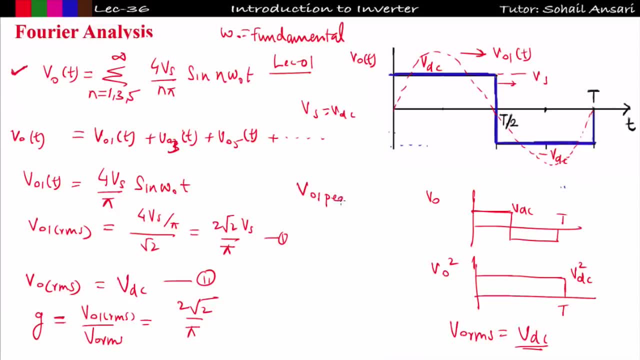 i will find the peak value of fundamental component v01 peak. it will be equal to 4 vs upon pi, which is greater than the peak value of supply voltage. this is my peak value of supply voltage. so 4 vs upon pi is greater than the supply voltage. 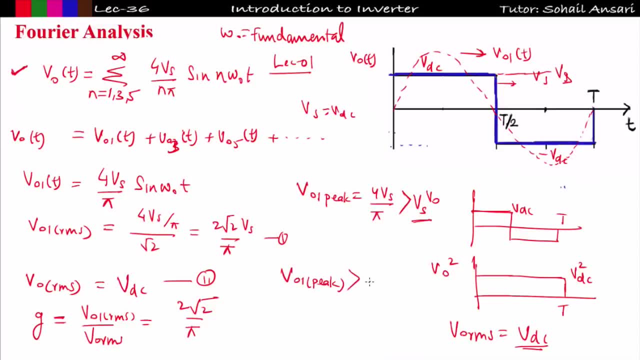 so i can say v01 peak is greater than v naught peak. i can say that. so this point you should understand and also write down your in your notes, that distortion factor of any square wave is independent of the peak value of output voltage. what do you mean by this? this means, if we will: 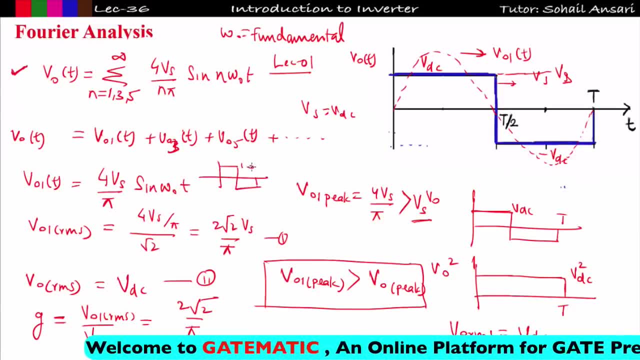 take the square wave having peak value 100, and if you will take the second square wave having peak value 50, okay, the distortion factor of this value is vz1 upon pi. this means v1 survived on the first, 여러분 og you understood. so now for the second distortion factor. the average of a means is: 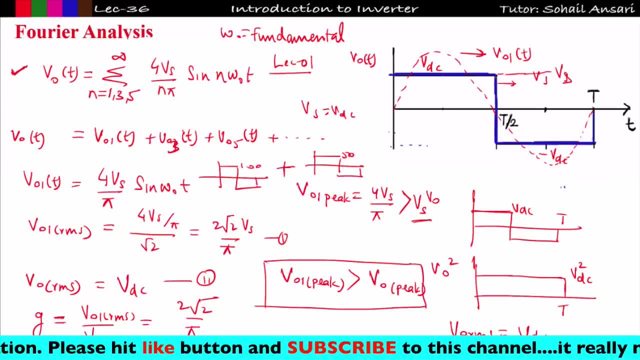 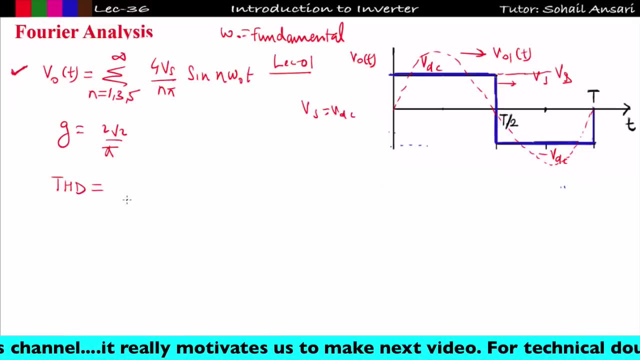 factor of both square wave will be equal to 2 root 2 upon pi. that is same, provided the time period will remain same. so i can easily find the thd, that is the total harmonic distortion. that is equal to 1 upon g square minus 1. so put the value of g, you will get thd is equal to 48.43 percent. 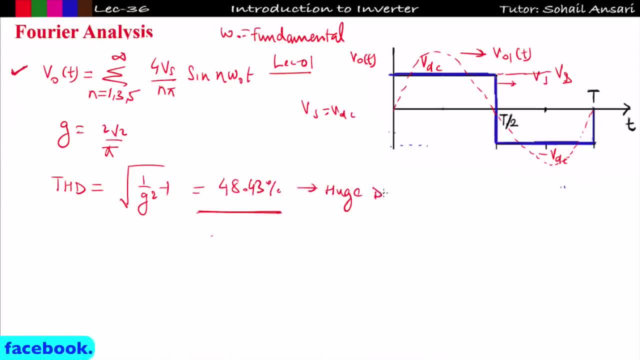 that is very huge, huge distortion. in a square wave there is very huge distortion, while according to ieee 519 1992 the thd must be less than 5 percent for household appliance. okay, and you are getting the thd 48.43 percent. so can you connect your load from those inverter whose thd is 48.43 percent? no, 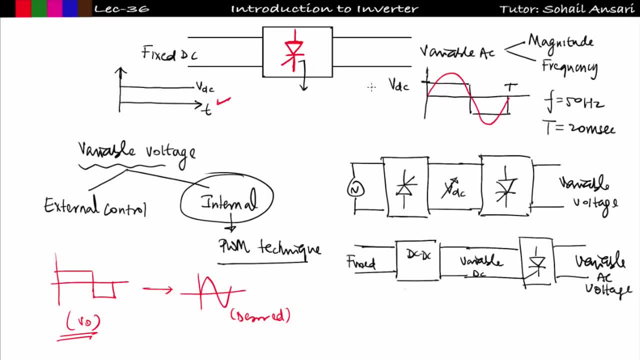 you can't. that's why i told you that we cannot connect this inverter directly to the real-time application. in order to connect this inverter, we need to insert a filter where we can connect this inverter to the real-time application. so, in order to connect this, 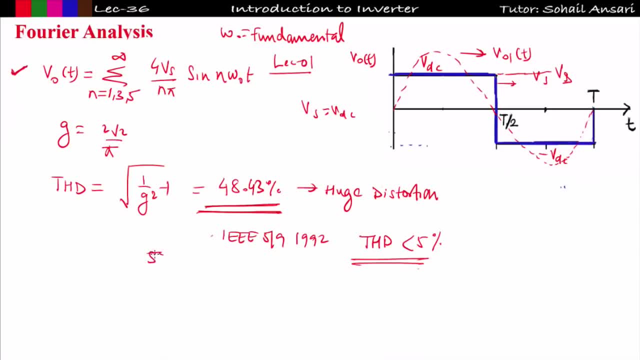 inverter which reduces the thd value and which can make the thd less than five percent. okay, and how will i decrease the thd- that is the another chapter that we will discuss later on- by using pwm technique and filter is not in gate syllabus. okay, so you should understand this all concept. 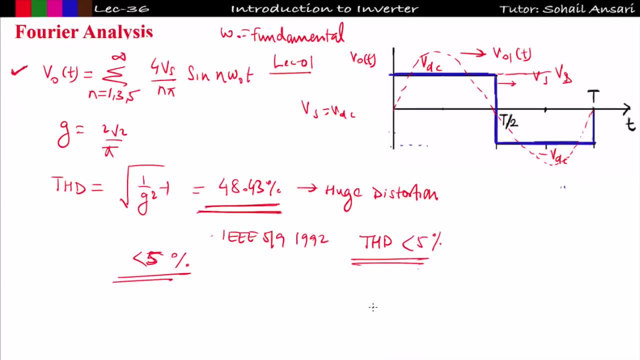 how we are doing the furrier and analysis of a square wave. how much a square wave is getting distorted from its fundamental. you should know these things because in every inverter lecture i will make the waveform and i will make the fundamental output voltage. so how the fundamental? 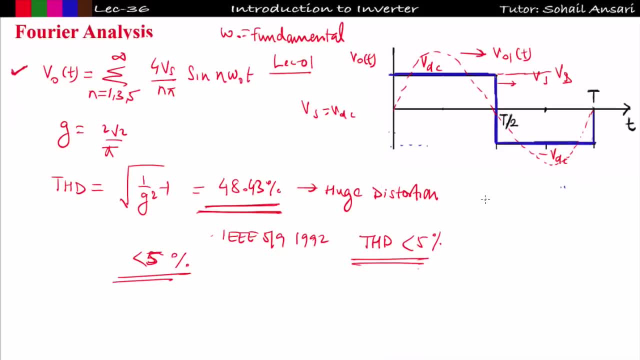 output voltage. i am getting by using four year series. these all things you should know and see. the fundamental: the peak value of fundamental output voltage v01, peak is greater than the peak value of output voltage that we have already seen. peak value of our fundamental output voltage force. 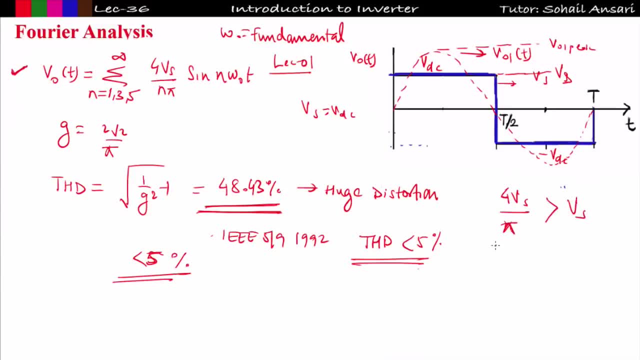 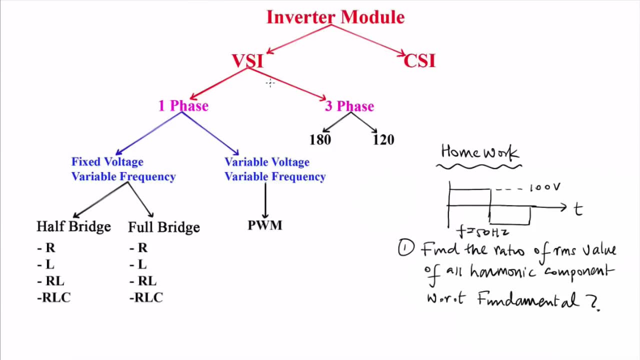 bs upon pi is greater than the vs right. so this much concept you should know before starting inverter. i created the inverter module like this: i divided in two parts vsi and csi, that is, voltage source inverter and current source inverter. in vsi there is single phase and three phase. again single phase. 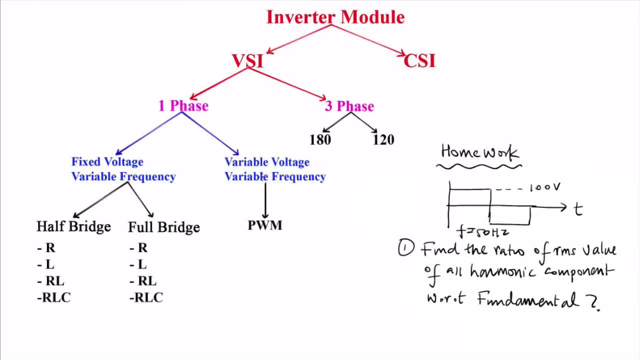 is divided in two categories: fixed voltage, variable frequency and variable voltage, variable frequency. this i will take in pwm technique and fixed voltage, variable frequency, again divided in two parts, that is half bridge and full bridge. in half bridge we will take a half bridge and full bridge r load, l load, rl load and rlc type of load. similarly, for full bridge we will take r load l. 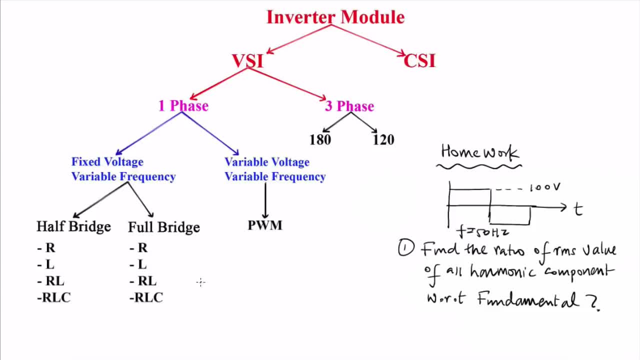 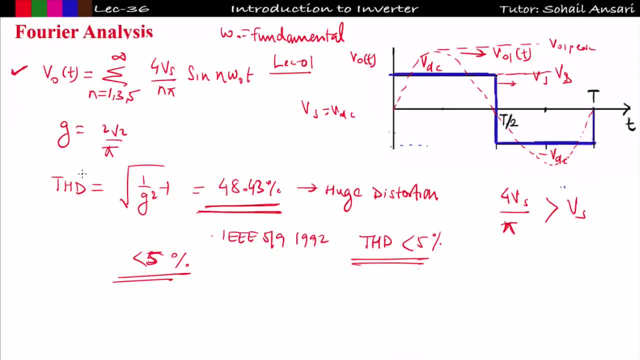 load, rl load and rlc type of load. so these all things we are going to discuss from next lecture, but before that you should know what is harmonics, why harmonics are undesirable, how to remove the harmonics. these all things we have discussed in lecture number one, so go through that before. 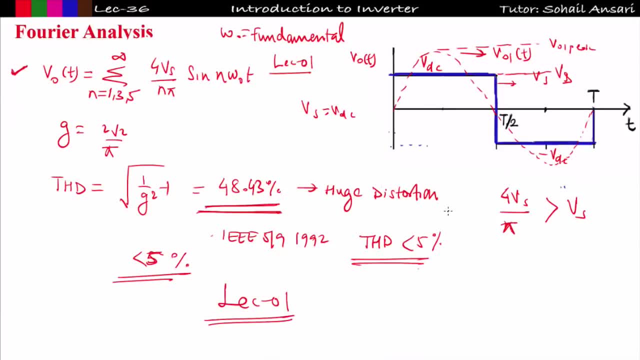 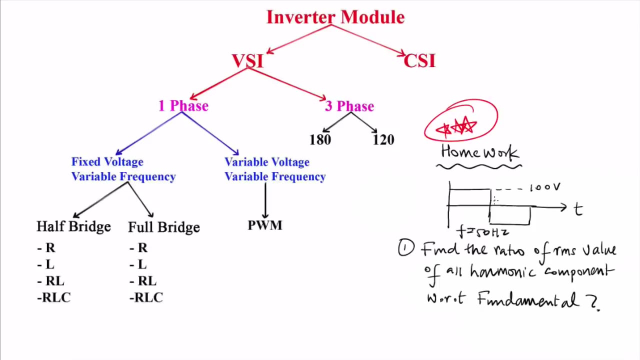 starting inverter. it will help you in understanding the concept. also, you should know how to draw the fundamental output voltage waveform, that is, the pure sine wave, how we draw this. you should know this. now, before closing this lecture, i am giving you one homework. this is the homework in which i have given you the 100 volt square waveform having frequency 50 hertz. 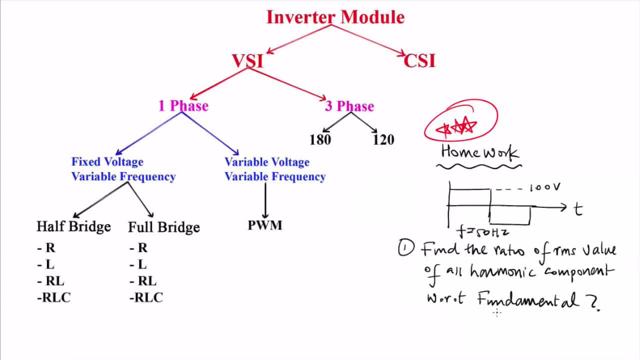 find the ratio of rms value of all harmonic component with respect to fundamental. we need to find the rms value of all harmonic component that is v03 rms plus v05 rms plus, so on upon with respect to fundamental, that is v01 rms. you need to find the ratio of this, find the solution and write down on your answer in youtube. 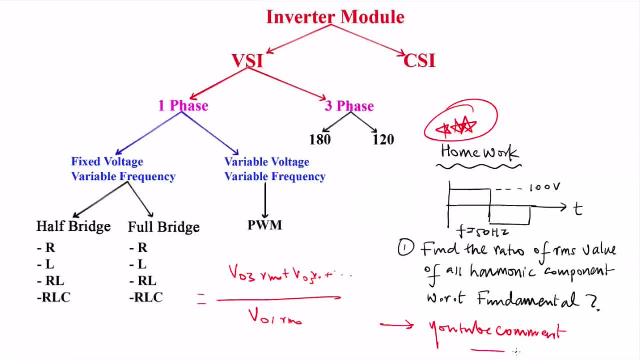 comment. in this way, we will get the feedback whether you have understood the concept or not. this is really important. if you will give me the feedback, then it will help me to make the next lecture. suppose you are getting the wrong answer, then i will include this homework in the next. 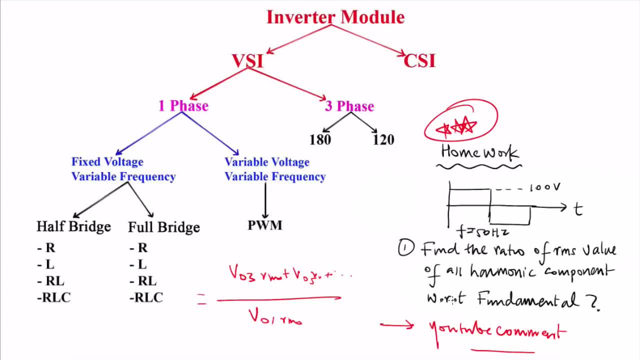 lecture and i will explain you where you did the mistake. so feedback is really important. please, guys, give me the feedback by liking or disliking the video or by commenting on this video. if you like this video, please subscribe to my channel and i will see you in the next lecture. bye, bye. 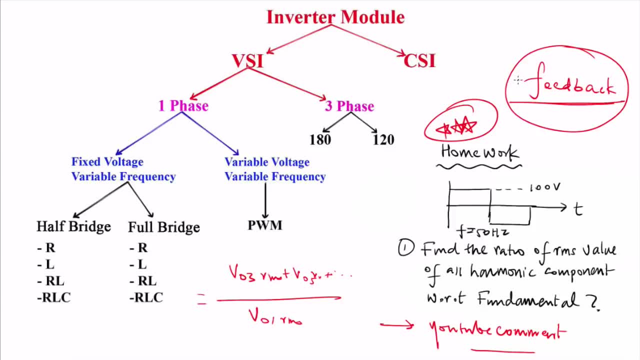 you should give me the feedback even if you are downloading the video. no problem, download the video, watch the video and, after watching the video, give me the feedback on youtube. comment, got it. that's all about this lecture. in the next lecture we will see single phase half bridge containing r.